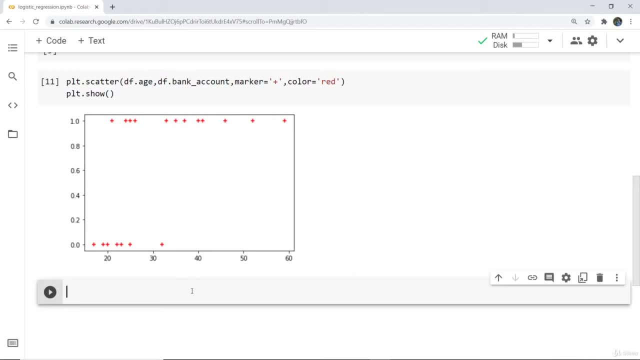 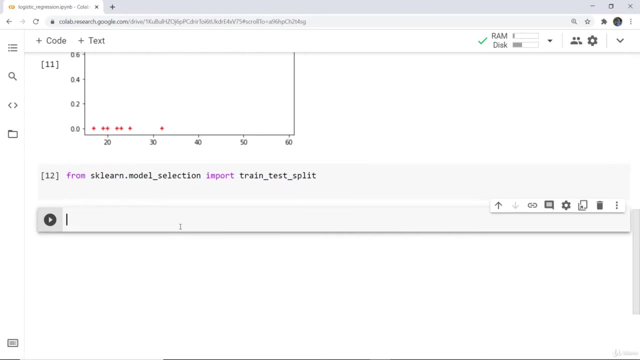 split the data and then we will perform the logistic regression. So for that: firstly we have to write like this: from sklearnmodelselection, import test, train data, that is, train and test split. Next you have to write the xtrain, xtest, ytrain and ytest and then you have to split on the 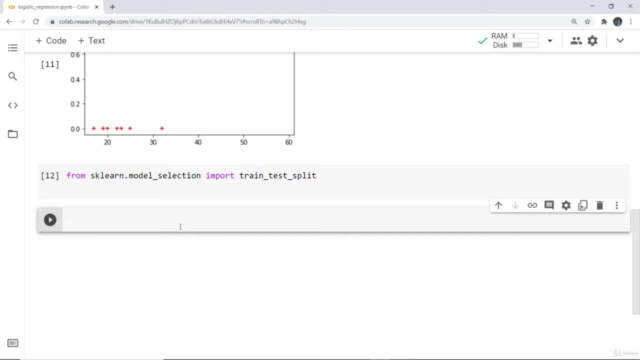 basis of it. So I'm splitting, like this age and the bank account. So you have to write like this: xtrain, xtest, ytrain, ytest equals to train test, split. and we are splitting df as age and next we are splitting dfbankaccount. 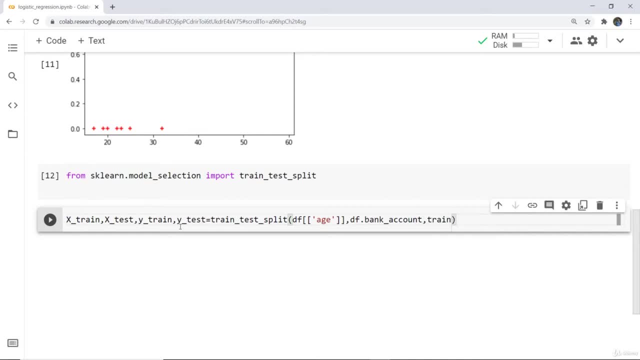 And here I am giving the train size also牛, and the trains size equals to 0.8. that means 80% of data I am using for training. and last, I will be using for testingho. So now I'm going to print xtest. that means 80% of data. 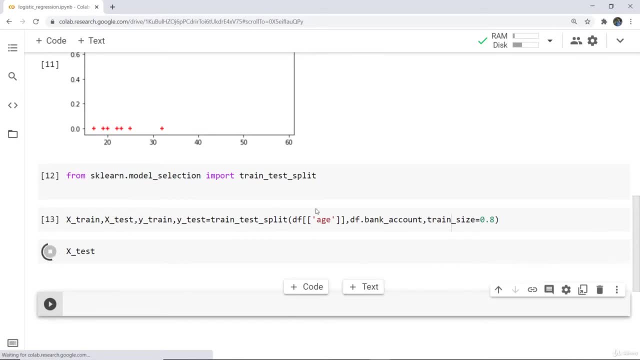 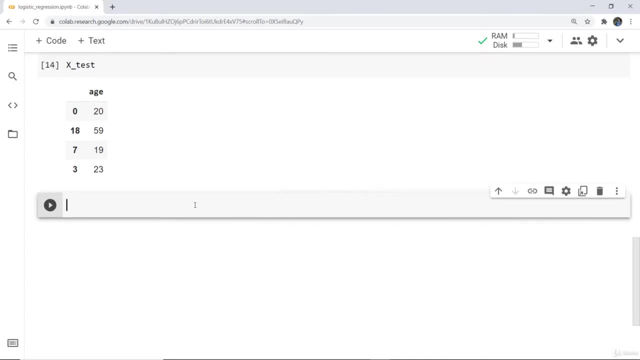 otros. So this is the data base content which is for testing. next, what we need to do: from sklearn linear model, we need to import logistic regression. so we write like this, just like we used to write for linear regression, also like sklearn dot linear model, import logistic regression. 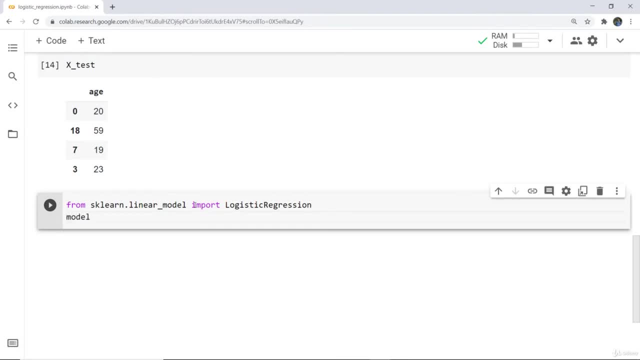 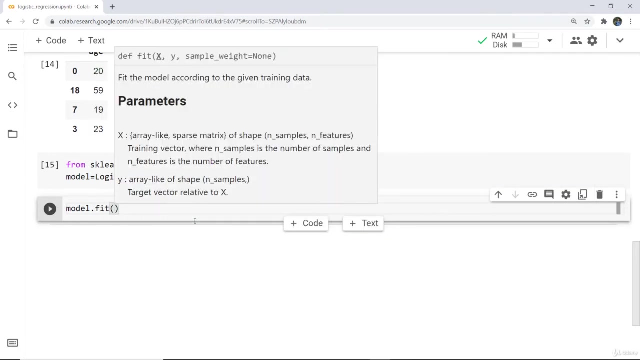 and then we need to name a model. equals to logistic regression. and then what we have to do? this: we have to fit the model, we have to train the model. so for that we have to write like this: model dot fit, and what we are fitting is fitting the. 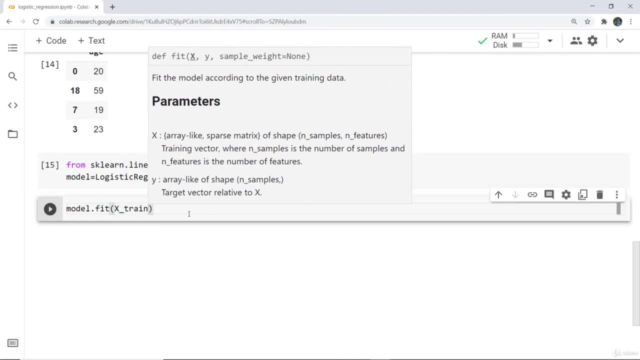 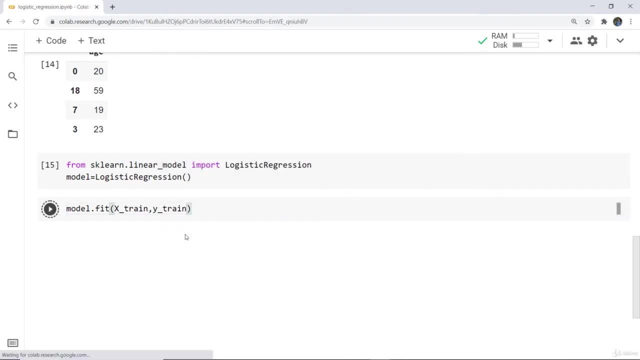 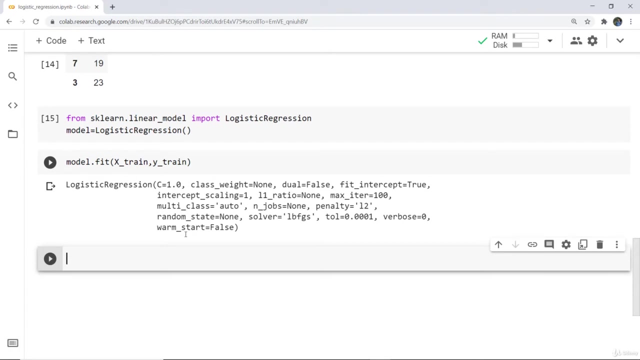 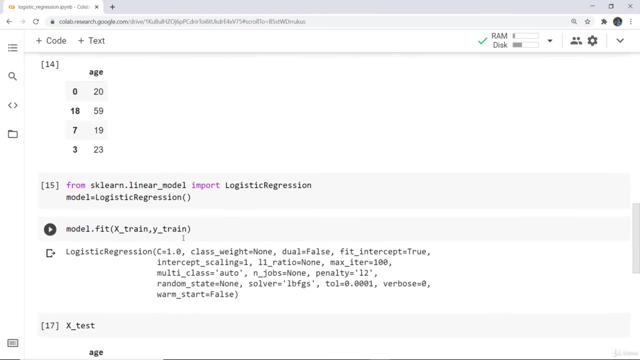 extreme and the Y train. so you can see here this is the logistic regression and all the state has been shown, the ratio and the max iteration and everything. and next we need to check the X test again. so this is the testing data which we have and earlier also it. 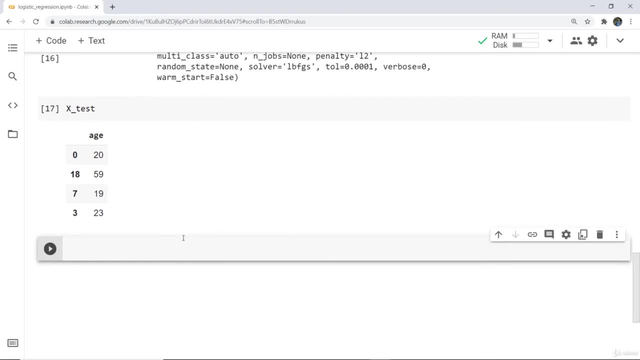 was same. so this has been fit to the machine. would it typically a machine? next we need to create another variable named Y, predicted, and in that we will have model dot predict X test. and now we're going to use this X test data to predict it. so we'll write like: 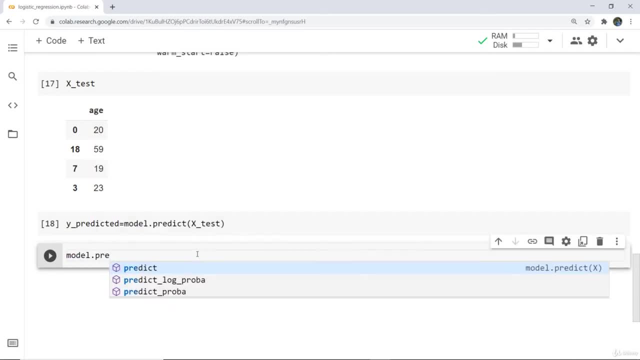 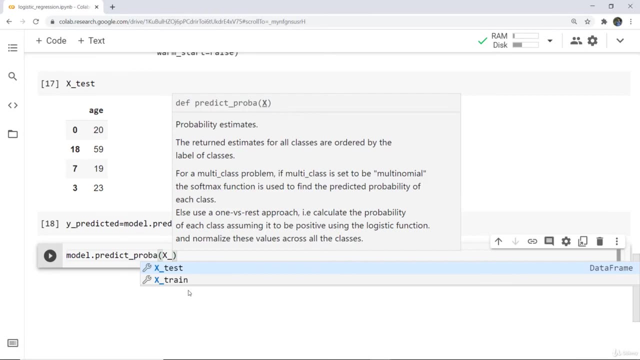 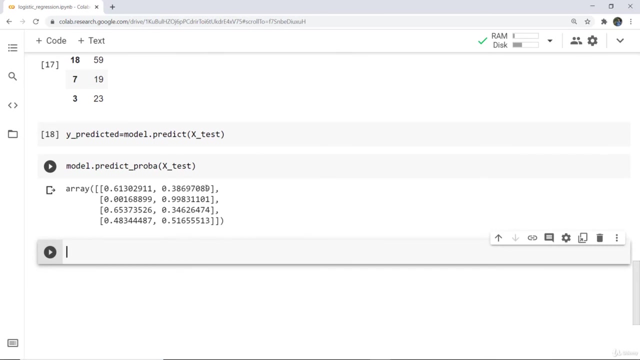 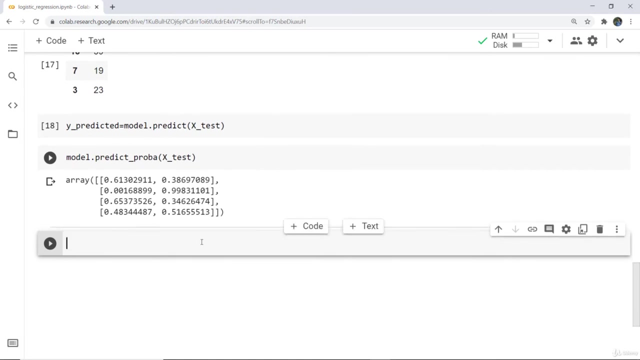 this model dot predict from. and then we are going to write X test here you can see that it has predicted the values of the X test data which we have given. similarly we can print the score also of the particular model. so for that we have to write like this model: dot score of X test, comma Y test. 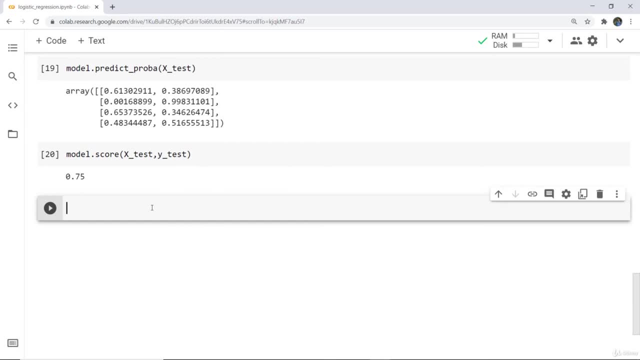 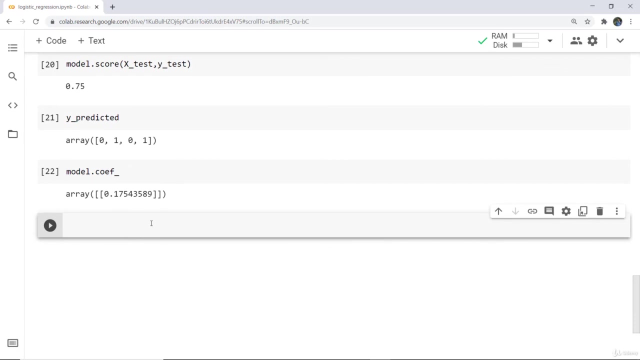 so this is the score of the model. next we can check Y predicted also. so this is the Y predicted array that has been displayed. and next, if you want to check the coefficient, then you can write like this: model dot coefficient. so this is the coefficient of the model. similarly, we can check for the intercept also. 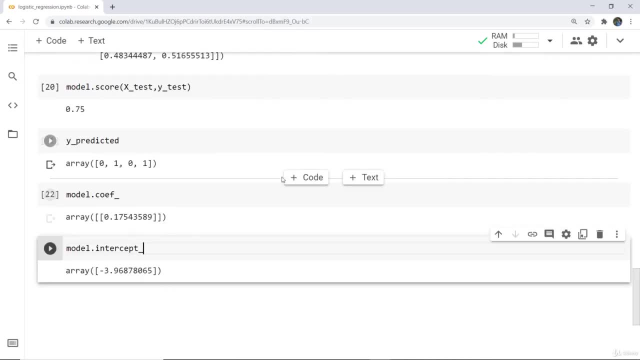 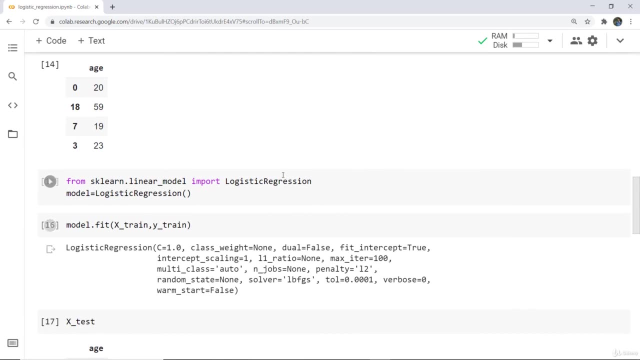 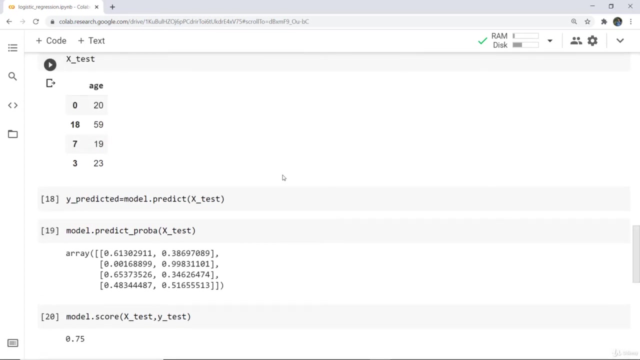 this is the intercept of the model. this is all about the logistic regression, in which we use the linear regression and from that we import logistic regression for training and testing data sets given to the model and then we can predict the score, the coefficient and the intercept. for more example of logistic regression: we will look into upcoming videos.